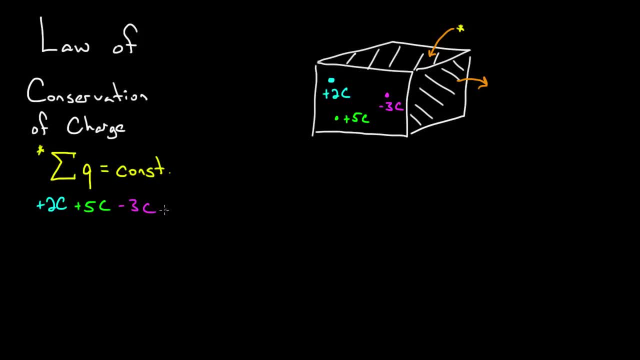 minus 3 coulombs, you'll get a number, and what that number represents is the total amount of charge in there, which is going to be: 5 plus 2 is 7, minus 3 is 4, positive 4 coulombs. 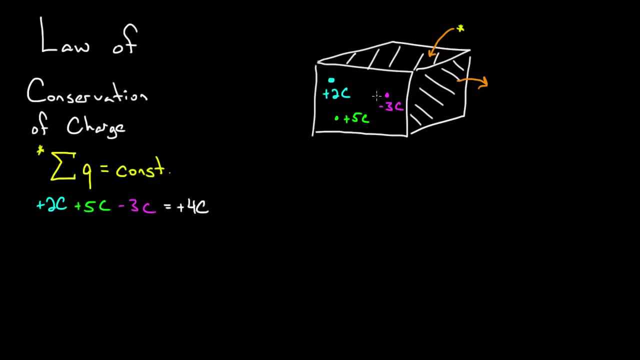 You ever open up this box, you're always going to find 4 coulombs in there. Now this sounds possibly obvious. You might be like duh. If you don't let any of these charges go in or out, of course, you're going to only find 4 coulombs in there. 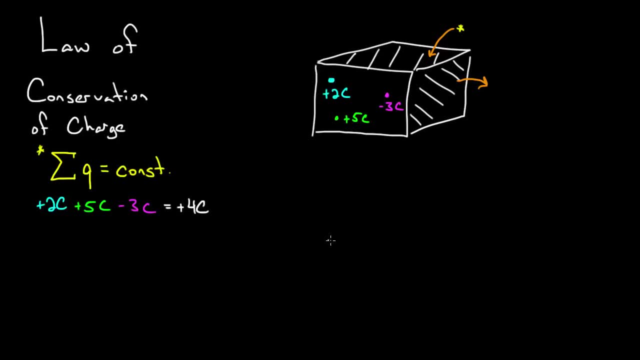 because you've just got these 3 charges, but not necessarily. Physicists know if you collide two particles, these things don't have to maintain their identity. I might end up with 8 particles in here at some later point in time. 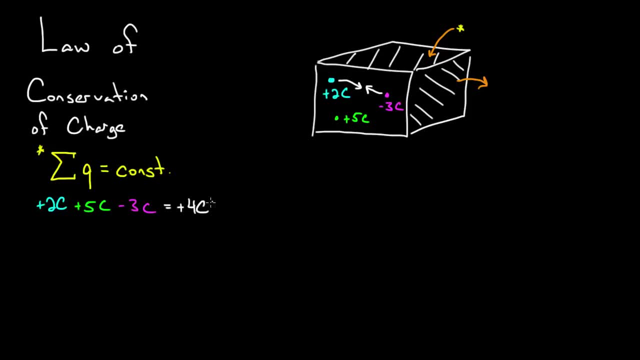 and if I add up all their charges, I'll still get 4.. That's the key idea here. That's why this is not just a frivolous sort of meaningless, trivial statement. This is actually saying something useful, because if these two, if these were protons- 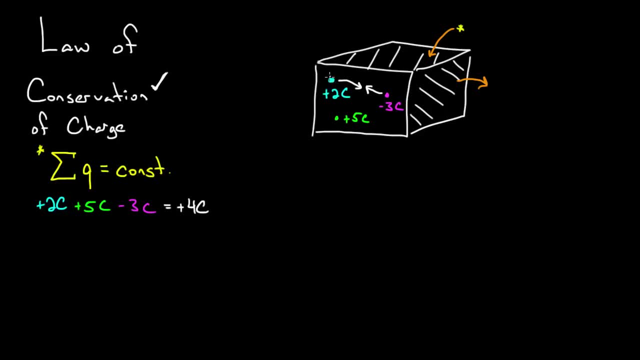 they're not, because this is a positive 2 coulomb and the proton has a very, very different charge. but for the sake of argument, say this was a proton. runs into some other particle- an electron, really fast. 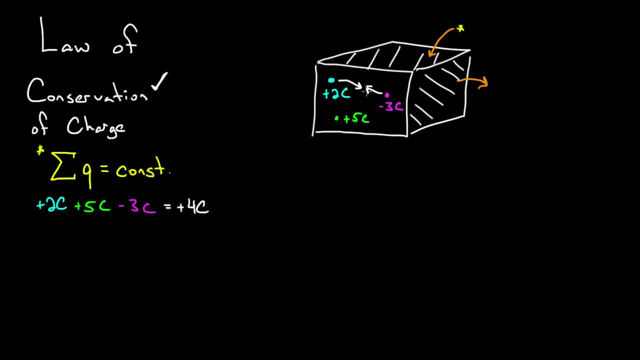 If there's enough energy, you might not even end up with a proton, an electron, You might end up with muons or top quarks, or, if this is another proton, you end up with Higgs, particles or whatever, And so at some later point in time- here's why this law is important and not trivial- 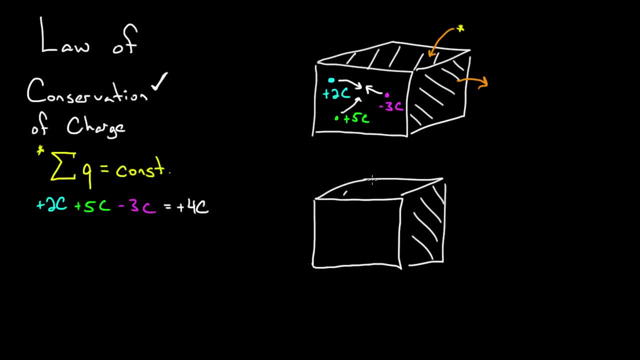 because if this really is closed up and the only stuff going on in there is due to these and whatever different particles they create at some later point in time, I may end up with like, say this one: it doesn't even have to have the same charge. 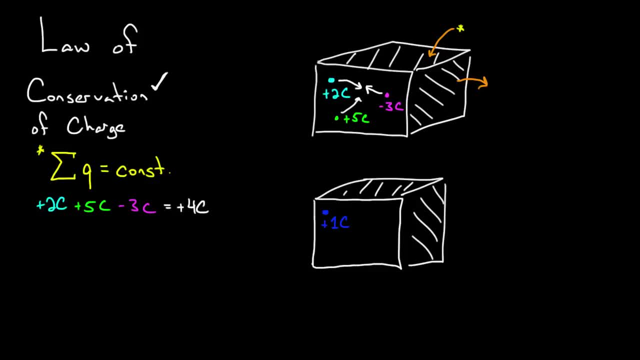 Maybe this one's positive 1 coulomb and I end up with a charge over here that has negative 7 coulombs. If these were fundamental particles, they would have charges much smaller than this. but to get the idea across, big numbers are better. 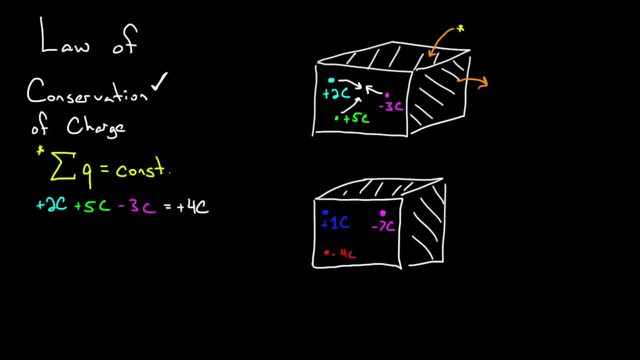 And let's say this is negative 4 coulombs. and then you end up with some other particle, some other particle you didn't even have there- None of these particles were there before- and some charge Q. Now we end up with these four different particles. 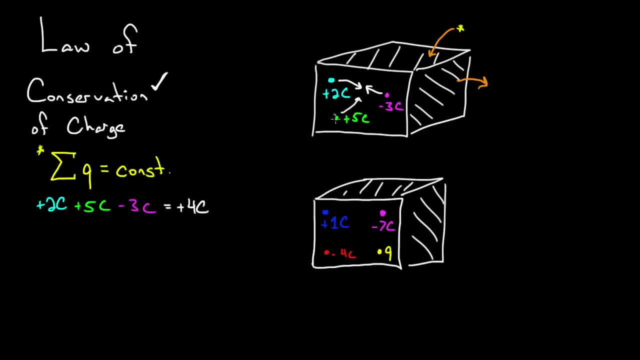 I don't know these combine. There was some weird reaction and they created these particles. What is the charge of this? Q? This is a question we can answer now and it's not even that hard. We know the charge of all the others. 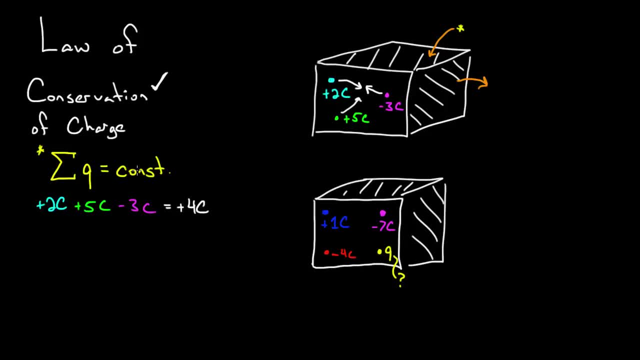 We know if you add up all of these you've got to add up to the same amount of charge you had previously, because the law of conservation of charge says if you don't let any charge in or out, the total charge in here has to stay the same. 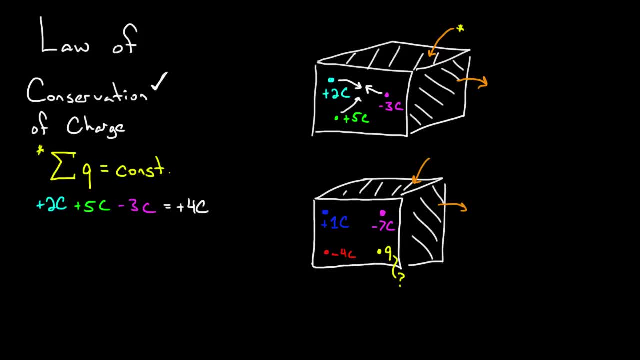 So let's just do it. We add them all up. We say that positive 1 plus negative 7 coulombs plus negative 4 coulombs plus whatever charge this unknown mystery particle is. we know what that has to equal. What does it have to equal? 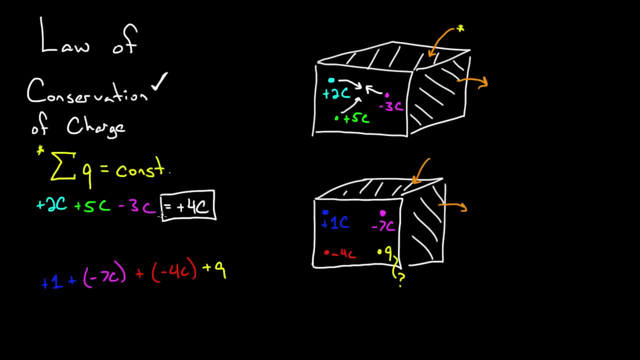 It has to equal the total charge, because this number does not change. This was the total charge before Positive 4 coulombs. That means it has to be the total charge afterward in there. That's what law of conservation of charge says. 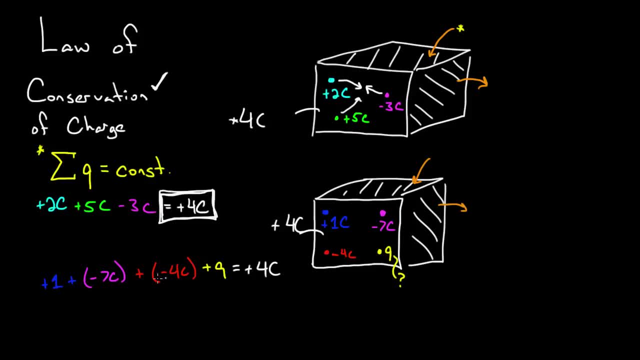 So that has to equal positive 4.. Well, negative 7 and negative 4 is negative. 11 plus 1 is negative 10.. So I get negative 10 coulombs plus. Oh, you know, these Qs look like 9s. 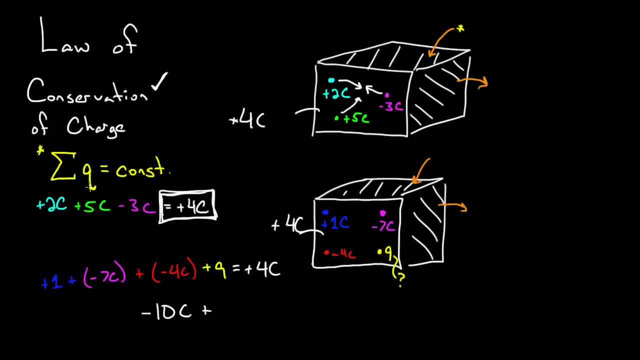 Sorry about that. This is law of conservation of charge. I might add a little tail. This isn't the law of conservation of 9s. So this is a little Q, This is a little Q. This is a little Q, not a 9.. 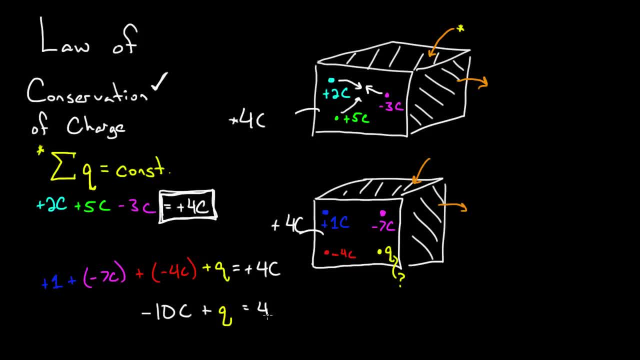 And so plus Q equals 4.. Now we know that charge has to have a charge of 14 coulombs in order to satisfy this equation. But you don't even really need a box. I mean, no one really does physics in a cardboard box. 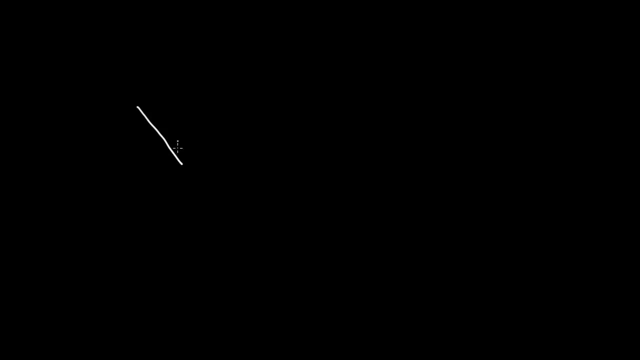 So let's say you were doing an experiment and there was some particle X, an X particle, and it had a certain amount of charge. It had say positive 3 coulombs. That would be enormous for a particle. But for the sake of argument, 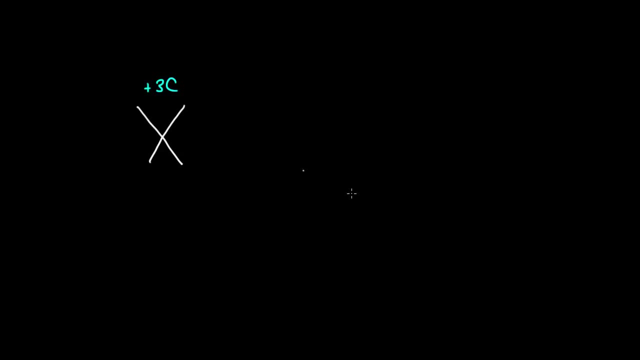 say it has positive 3 coulombs. Well, it decays. Sometimes particles decay. They literally disappear, turn into other particles. Let's say it turns into a Y particle and a Z particle. Just give them random names And you discover that this Y particle 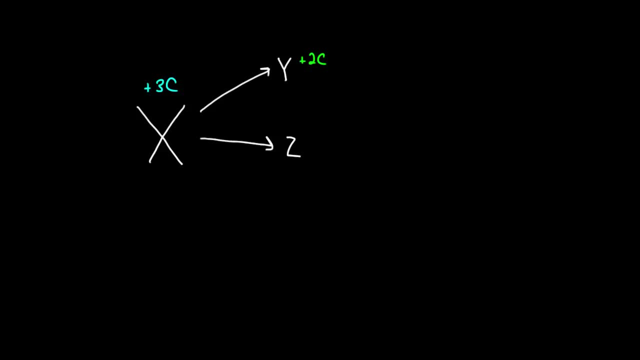 had a charge of positive 2 coulombs And this Z particle had a charge of negative 1 coulomb. Well, is this possible? No, this is not possible. If you discover this, something went wrong Because this side over here. 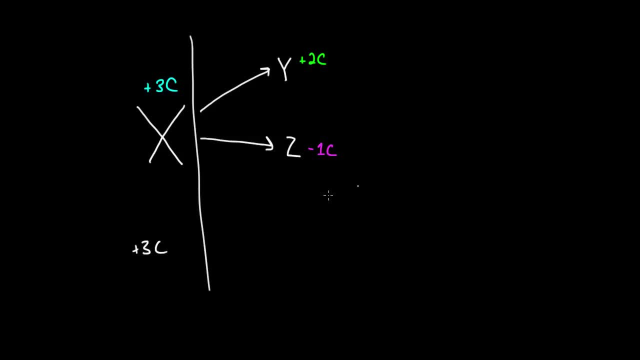 you started off with positive 3 coulombs. Over here you've got to end up, according to the law of conservation of charge, with positive 3 coulombs, But positive 2 coulombs minus 1 coulomb. 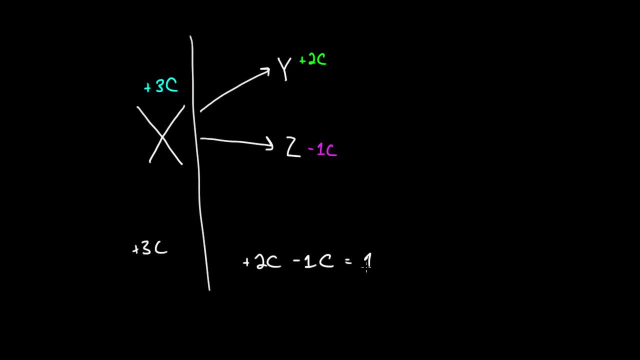 that's only 1 coulomb. You're missing 2 coulombs over here. Where did the other 2 coulombs go? Well, there had to be, There had to be some sort of mystery particle over here that you missed. 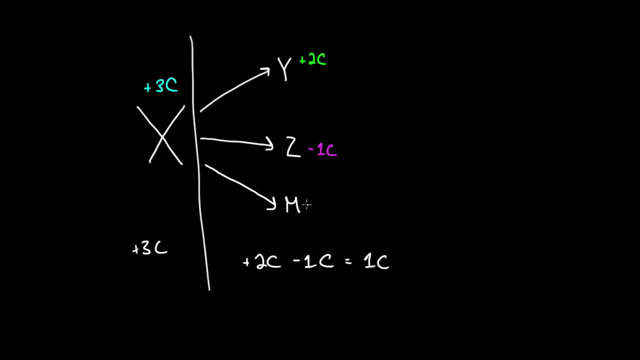 Something happened. Either your detector messed up or it just didn't detect a particle that had another amount of charge. How much charge should it have? This whole side's got to add up to 3.. So if you started off with 3,, 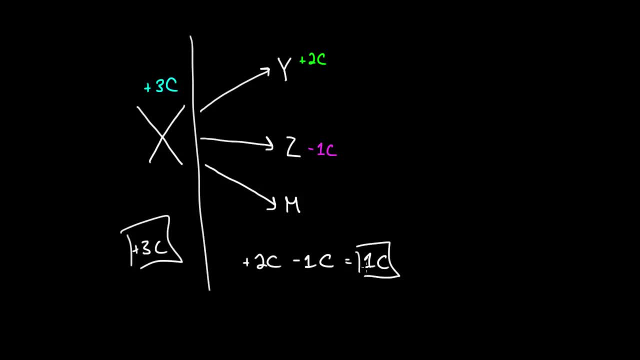 over here. these 2 together, Y and Z, are only 1 coulomb. That means the remainder, the 2 coulombs. the missing 2 coulombs has to be here. So you must have had some particle. 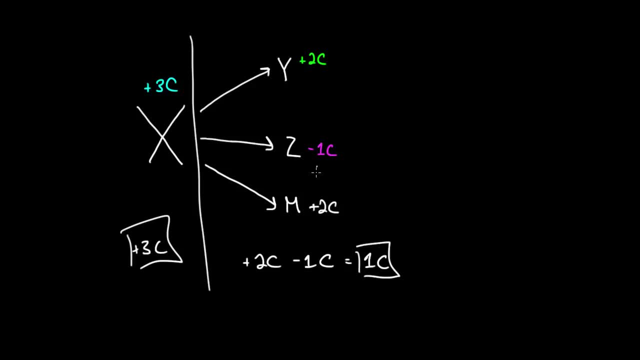 or some missed charge that has positive 2 coulombs. Is that another Y particle? Maybe That's why physics is fun, Maybe it is now. Maybe you missed another one. Let me ask you this. So let's say we get rid of all these charges. 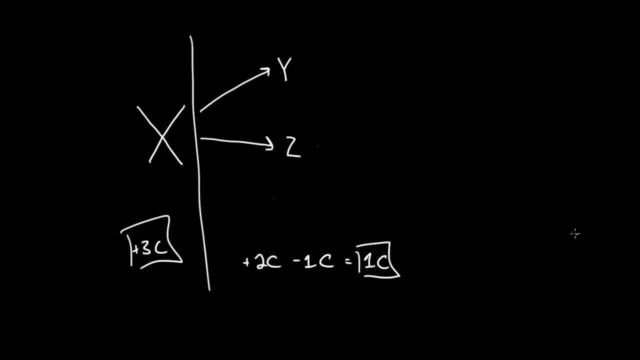 Here's one that freaks people out sometimes. Take this. Let's say: this had no charge. No charge, It was uncharged. You had some particle with 0 coulombs. Is it possible to end up with particles that have charge? Yeah, it can happen. In fact, if you have a photon that has no charge, It's possible for this photon to turn into charged particles. How is that possible? Doesn't that break the law of conservation of charge? No, but you've got to make sure. 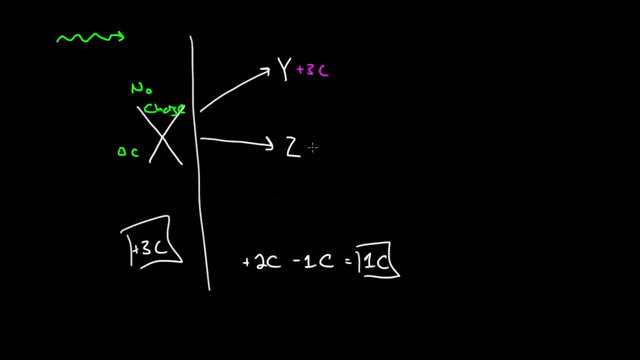 that whatever charge this gets- say positive 3 coulombs, this one's going to have to have negative 3 coulombs, so that the total amount of charge over here is 0 coulombs, just like it was before. So this is weird, but yeah.